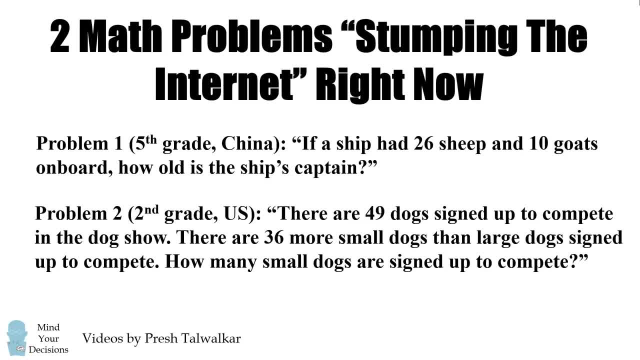 The second problem was given to second graders. in the US There are 49 dogs signed up to compete in the dog show. There are 36 more small dogs than large dogs signed up to compete. How many small dogs are signed up to compete? I'm going to go over each of the headlines of each of these problems. 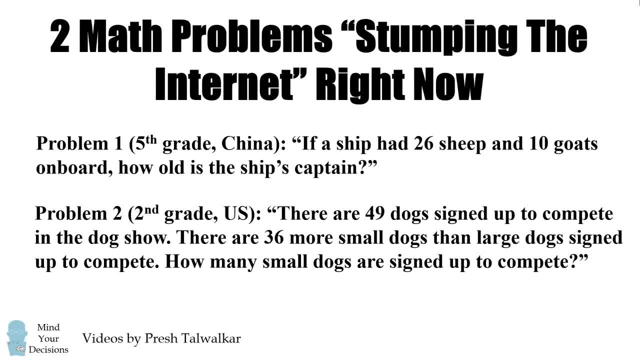 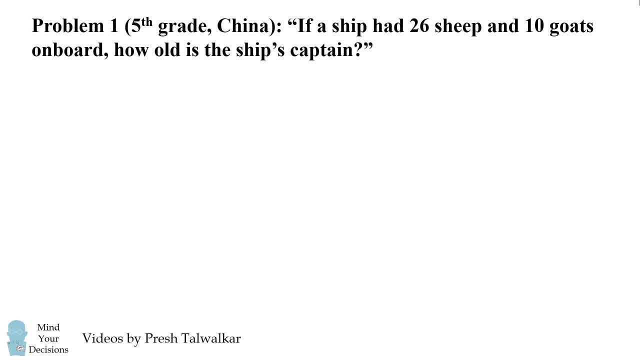 and then go over a little bit of discussion about each problem. So let's start out with the first problem, As this all begins. let's start off by asking the question we don't often hear about. Here is a sample of the headlines generated all over the world. 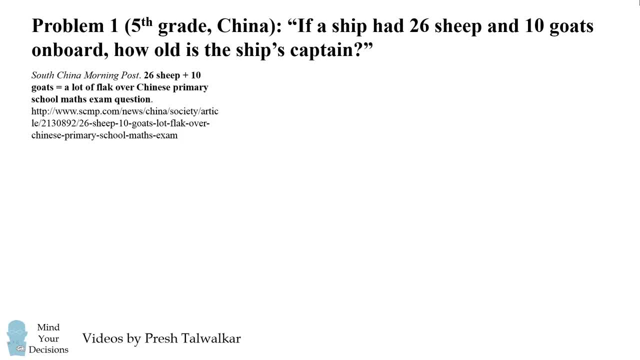 From the South China Morning Post: 26 sheep plus 10 goats equals a lot of flak over Chinese primary school math exam question From RT: 26 sheep, 10 goats and ship's captain- unsolvable math problem puzzles Chinese students. 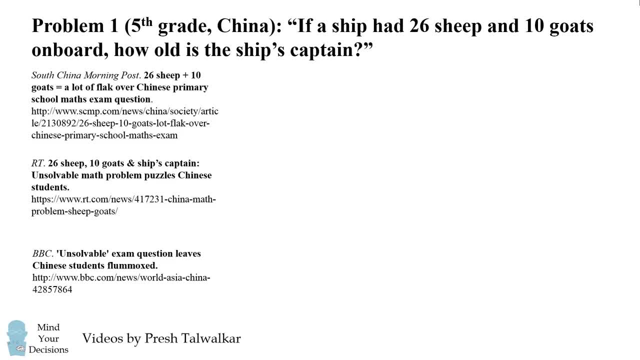 From the BBC: unsolvable exam question leaves Chinese students flying機 results every day. There are signs, only signs mixed. From the Washington Post: this Chinese math problem has no answer. Actually, it has a lot of them. And from: 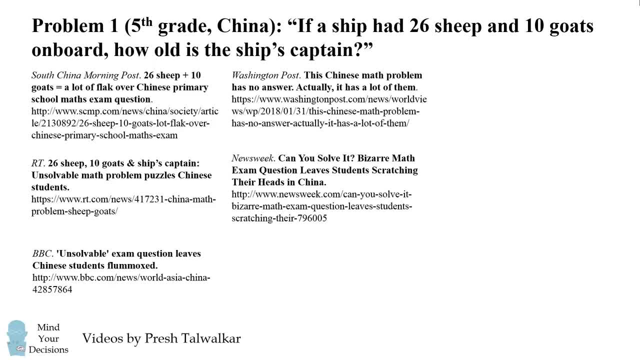 Newsweek. can you solve it? Bizarre math exam question leaves students scratching their heads in China. So there actually was an official response. They said the question was not a mistake. It was meant to be open-ended, to encourage critical thinking. So how might you estimate how? 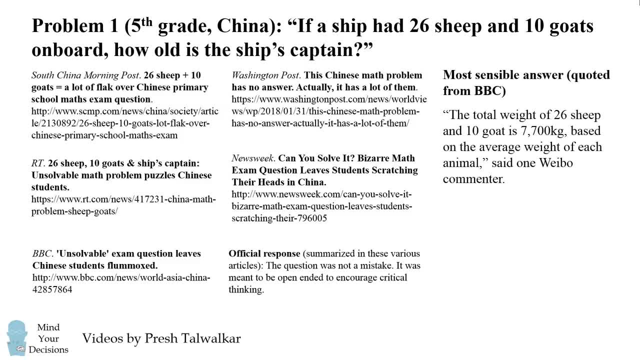 old. the ship's captain is The most sensible answer I saw that was quoted in the BBC comes from someone who's commenting on Weibo. The total weight of 26 sheep and 10 goat is 7,700 kilograms, based on the average weight of. 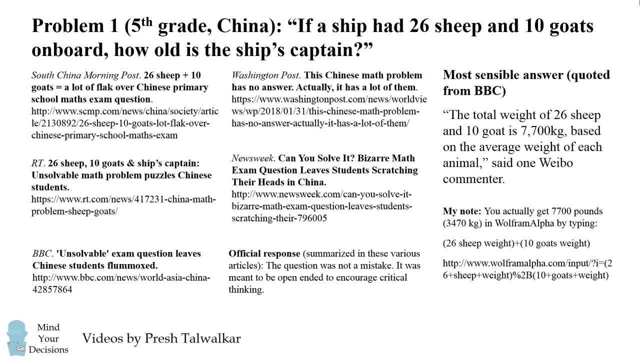 each animal. Now I did a little bit of fact-checking and if you type in 26 sheep weight plus 10 goats weight into Wolfram Alpha, the computational search engine, you actually get 7,700 pounds, which is approximately 3,470 kilograms. So I'm 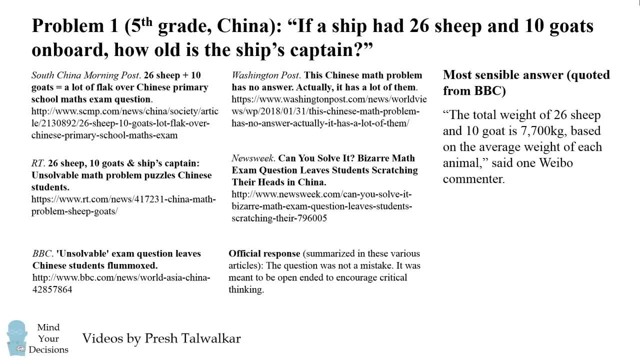 not sure exactly where they got that number of 7,700,, but let's just go with it for the rest of the answer. In China, if you're driving a ship that has more than 5,000 kilograms of cargo, you need. 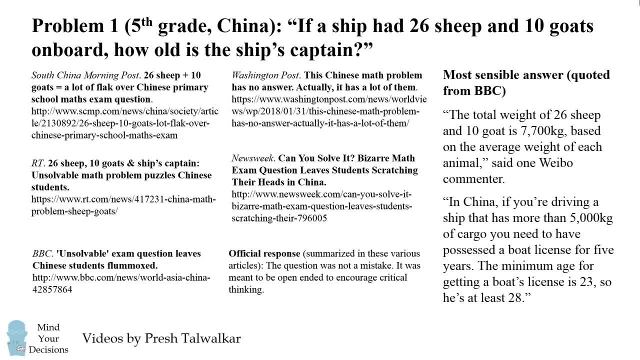 to possess a boat license for five years. The minimum age for getting a boat's license is 23,, so he's at least 28,, or the ship captain is at least 28.. So there could actually be some interesting critical reasoning from this problem. but 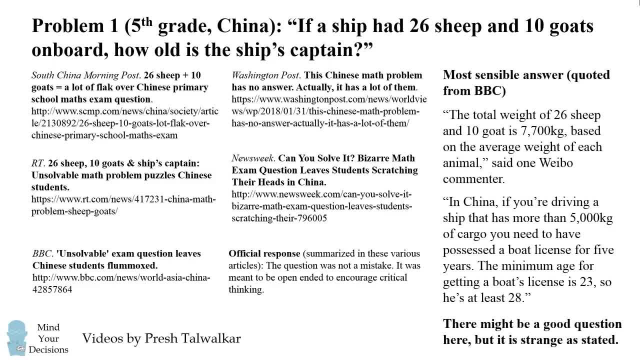 to give it to fifth graders as a math question. it just seems a little bizarre, and so that's what generated all these headlines around the world, And it's very bizarre that the official answer was that this was not a mistake and it was. 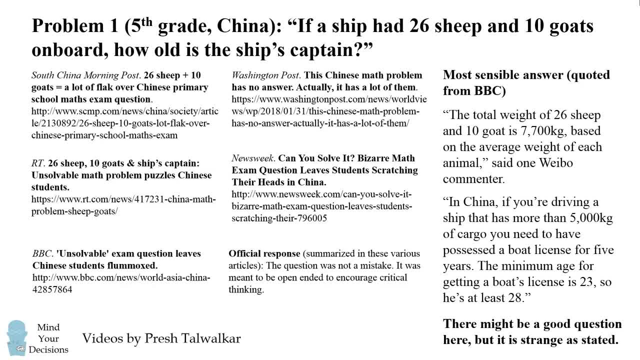 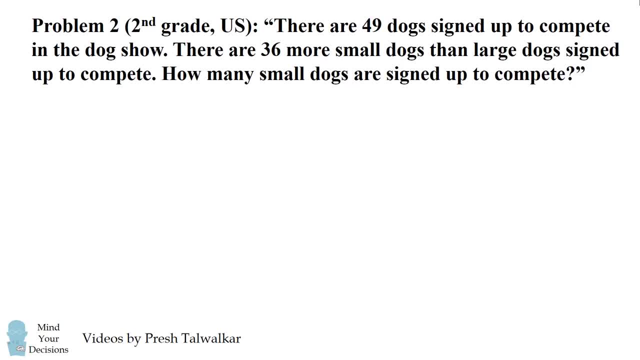 meant to encourage this kind of critical thinking. So now let's move on to the second question. So there are 49 dogs signed up to compete in the dog show. There are 36 more small dogs and large dogs signed up to compete. How many small dogs are? 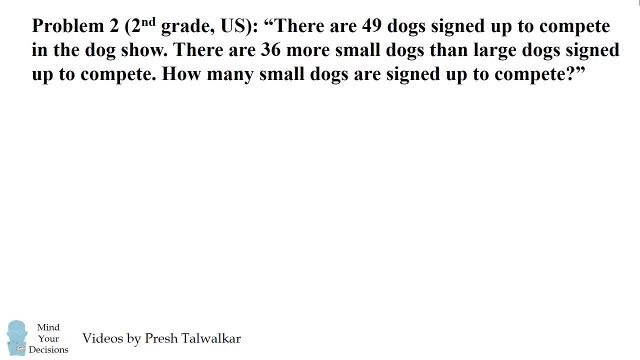 signed up to compete. So this seems like a standard algebra problem, but it also generated a ton of headlines. PopSugar reported the internet is losing its over the second-grade math problem. The Daily Mail mother is left stumped by her seven-year-old 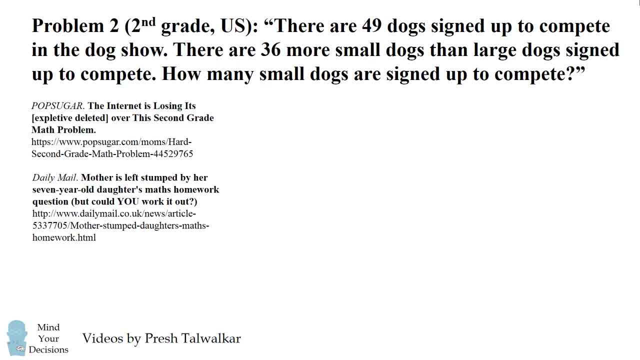 daughter's maths homework question, but could you work it out From the New Zealand Herald: math question for seven-year-olds breaks the internet From Forbes. this is actually from contributor Kevin Knutson, who has a podcast: My Favorite Theorem, which I encourage you. 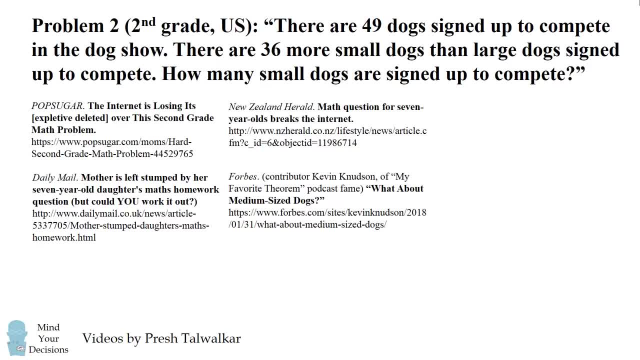 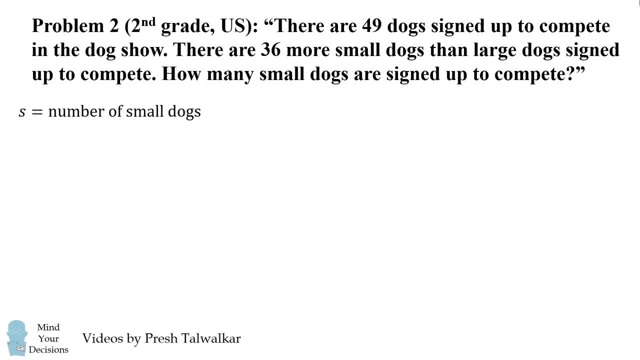 to check out, He wrote an article: What about medium-sized dogs? So how can we solve this problem? Let s denote the number of small dogs and let l denote the number of large dogs, As there are 36 more small dogs than large. 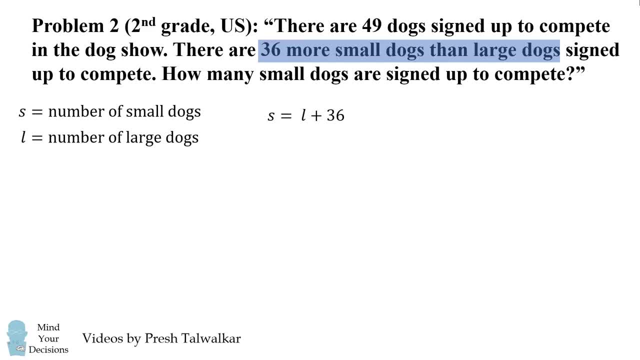 dogs, we have the equation s equals l plus 36.. There are 49 dogs signed up in total, so s plus l equals 49.. We then take the second equation and substitute: s is equal to l plus 36.. So we get the.